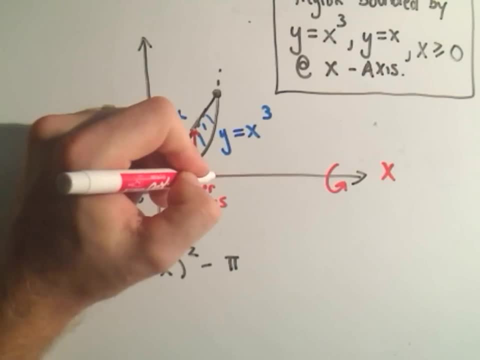 Well, again, I do the same thing. I start at the line I'm rotating about, and I draw it until it just touches the region. 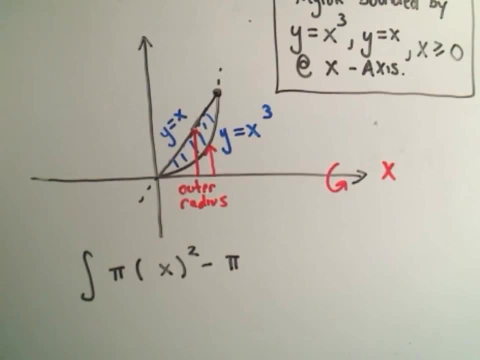 And then in this case, I think, well, what curve is it hitting? The curve that it's hitting in this case is x-cubed. But again, I have to square that. 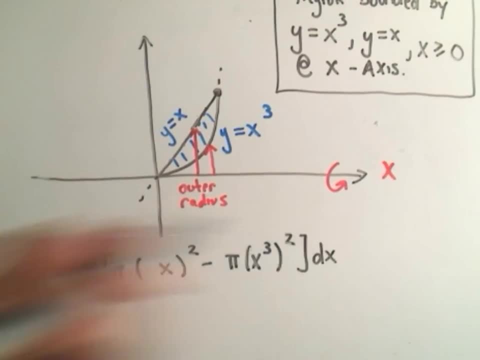 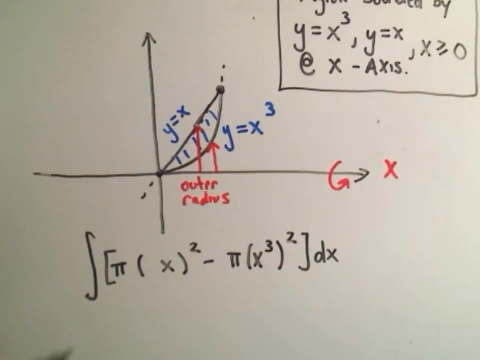 So we're integrating this with respect to x. So that means the limits of integration are going to come from the x-axis. Well, the smallest x-coordinate that we're using here is 0. Well, to get the largest one, in general, you have to set these things equal to each other and then solve. 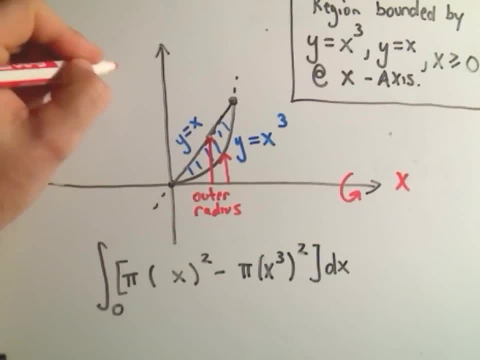 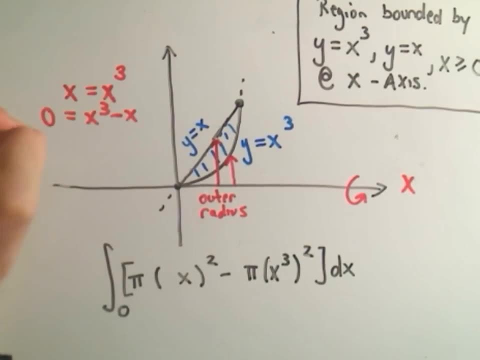 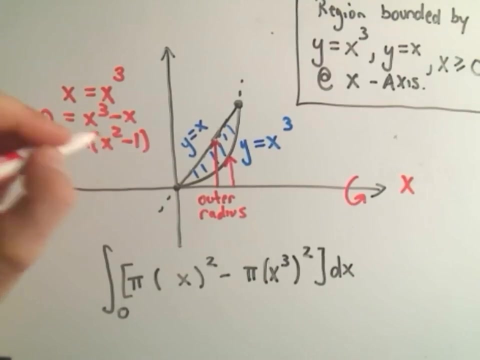 I mean, you can guess probably the value. But again, just a little bit of algebra refresher. Set them equal, then make one side 0. We could factor out an x. We would get x-squared minus 1. If you factor x-squared minus 1, we would get the solutions x equals 0 from the first part, and then positive and negative 1. And again, if you kept graphing, these things would cross over here at negative 1. So that's why we're getting all three solutions. 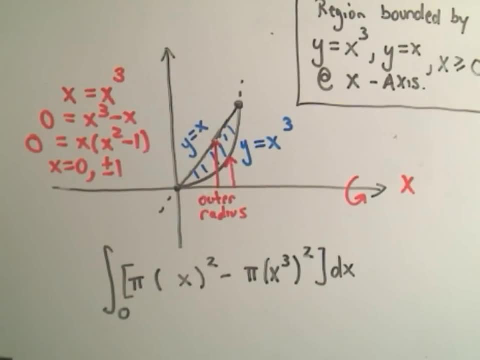 But clearly, in the first quadrant, this will be the x-coordinate of positive 1 where they're hitting. So this would be 1, 1. The y-coordinate's irrelevant. In this case, all we need is the x-coordinate. 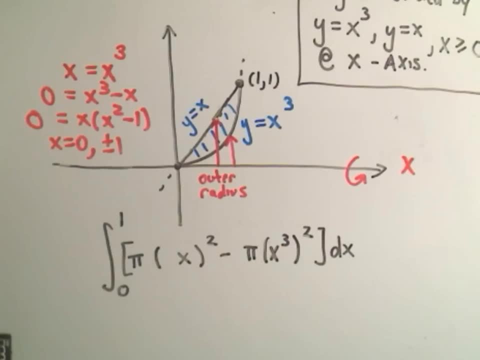 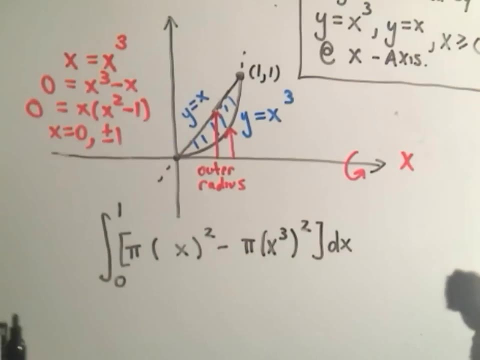 And that's now the setup to calculate the volume. So remember, volume should always be positive. So if this doesn't work out to be something positive, certainly you've done something wrong. So let's just go ahead and integrate this in one fell swoop. We could factor the pi out. 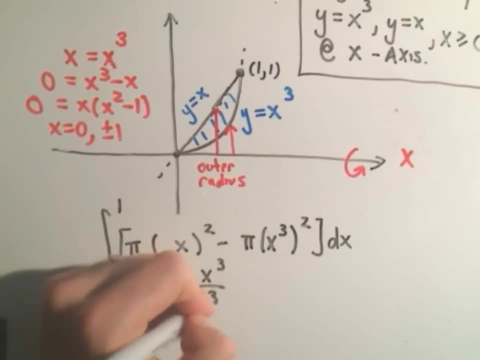 I'll get x-squared. If I integrate that, I'll get x to the third over 3. 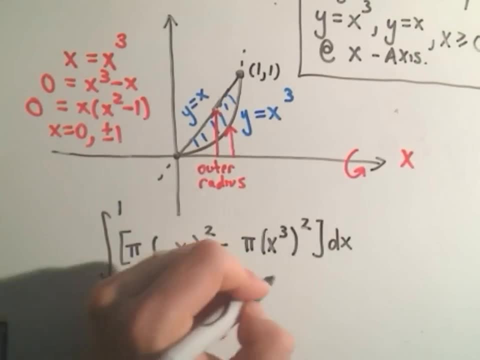 Again, I factored the pi out. I would have x to the sixth. 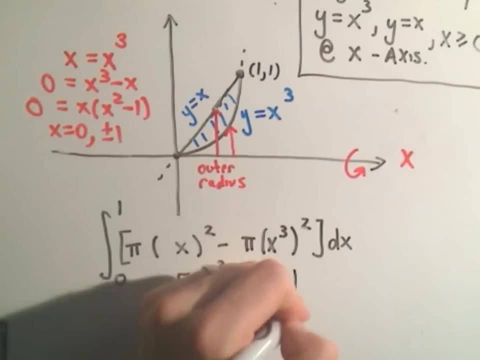 If you integrate, that'll be x to the seventh over 7 from 0 to 1. Well, all we have to do now is plug our limits of integration in. If you plug 1 in, you'll get 1 third minus 1 seventh.